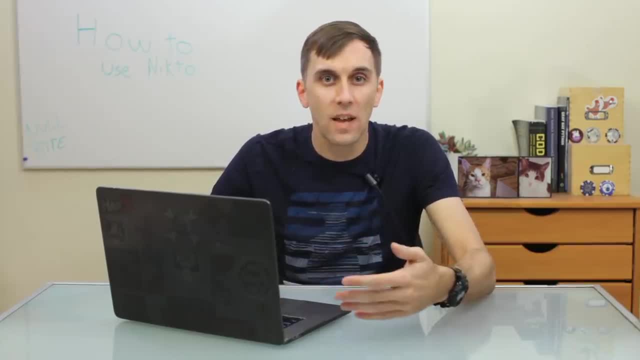 And what this means is we find a vulnerability that somebody else has not only exploited, but created a tool that will automatically do whatever it is we're trying to do, So we can basically put in some code or do something else that otherwise wasn't intended for us to be able to do on that device. 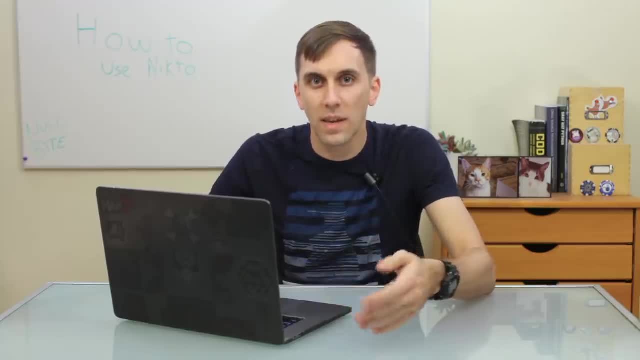 Now this is kind of the cycle of Nikto. We find something, we put it through Nikto and through that active scan we find a better way of attacking than maybe some much longer, more invested scheme we would have to pull off otherwise. 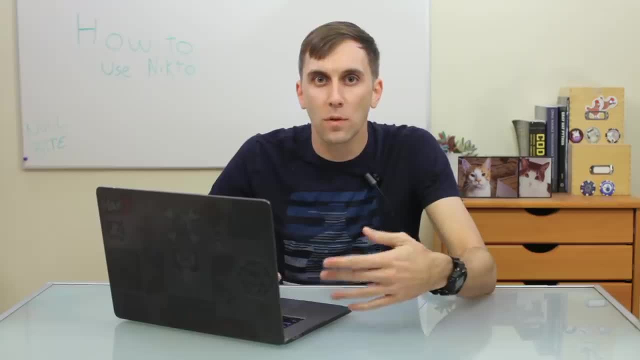 This is the way that we can use Nikto to be able to make an attack much more cheap and effective. So, in general, if you're looking to do an attack, it's worth your while using a vulnerability scanner, and Nikto is one of the easiest. 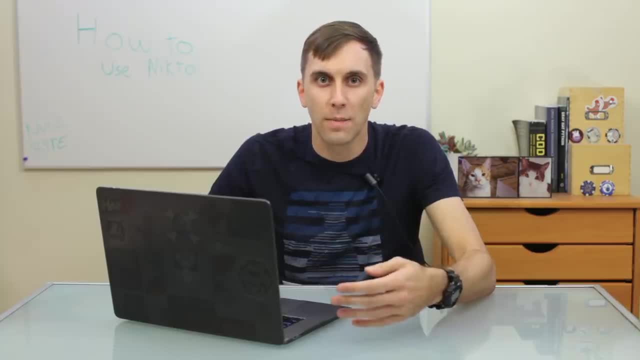 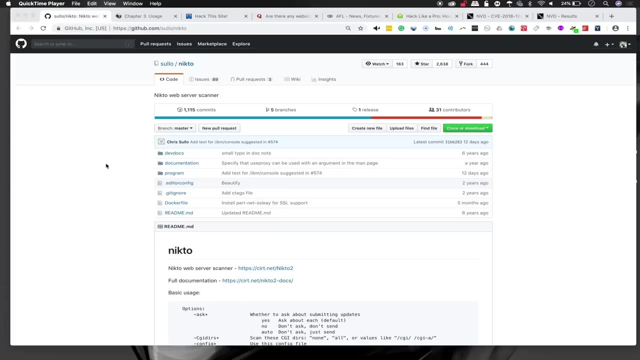 If you're looking to do this, you can simply download it from the GitHub repository. So in order to begin, you'll just need to download that first. Once you have that, we can get started. Now, the first step to installing Nikto is to go to the GitHub repository. 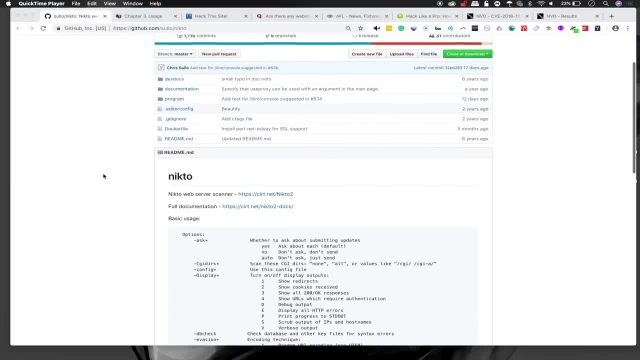 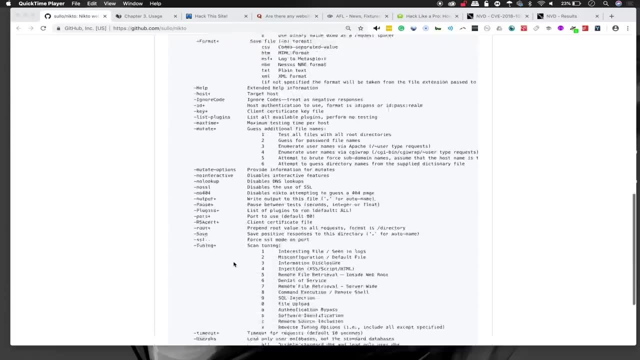 and here you can find a lot of things- to information, such as the full documentation that will be useful if you want to truly master this web scanner. Now, here you can see a full list of all the options, which is, again, very useful. 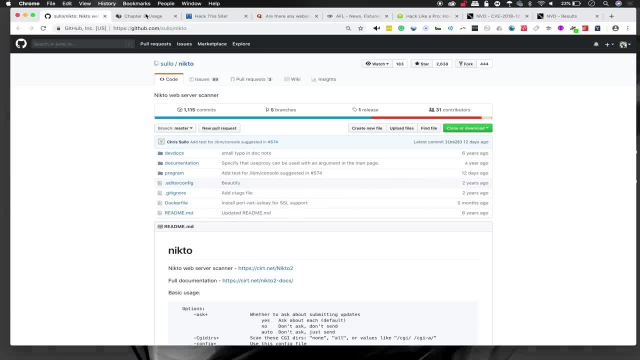 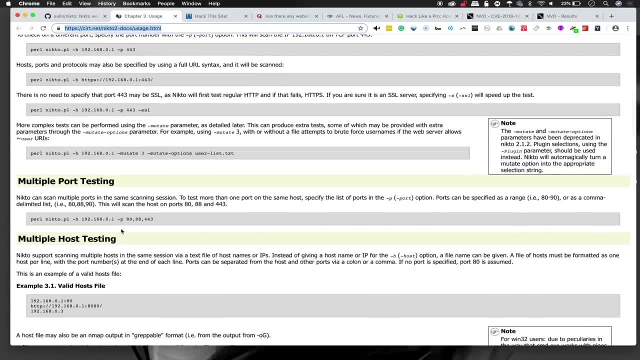 but really the good stuff is on the full documentation and you can even see the chapter on basic usage here includes some really interesting use cases like multiple port testing, where you can test for, let's say, you suspect that the the web server is running on a non-standard port, so maybe port 81 or 88,. 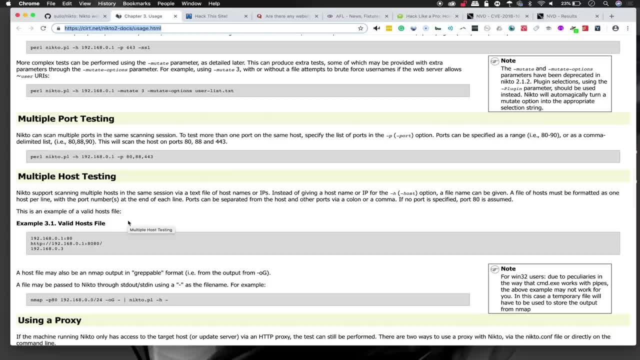 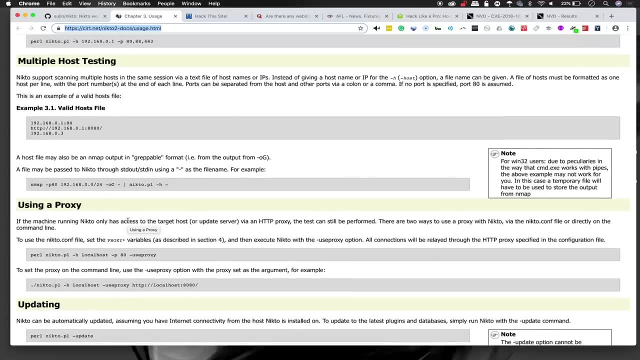 multiple host testing, meaning we can test a bunch of different hosts all in the same go and we can also use a proxy, So that allows us to get around. maybe restrictions on us scanning the target if we've been blacklisted, for example. 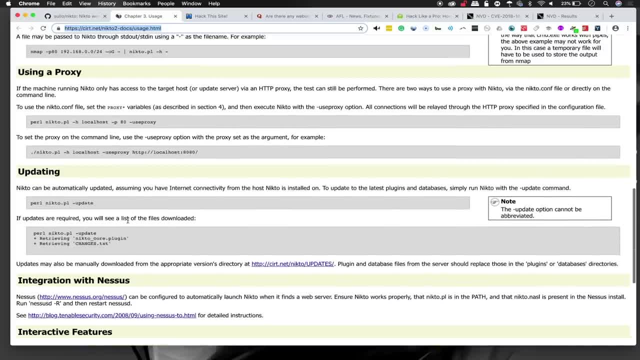 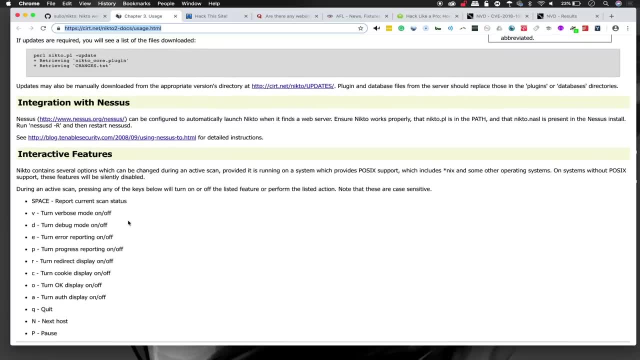 or if we just don't want to be attributed as the one who's actually doing the scanning. You can also see that there's some integration with Nessus, which is a web application security vulnerability scanner, and then you can also do some output compatibility with Metasploit. 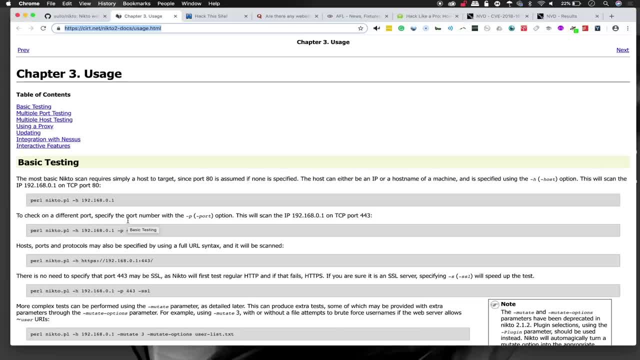 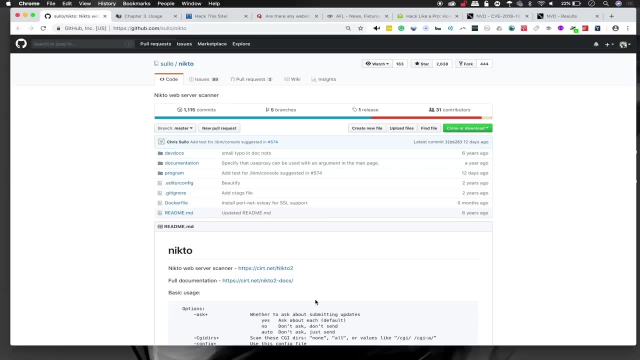 which allows you to take the vulnerabilities that you discover and pair them with exploits, So that's all really cool. In general, though, if you want to install this, you can go ahead and install it from the GitHub repository, but if you are using Kali Linux, you can just type apt, install nikto. 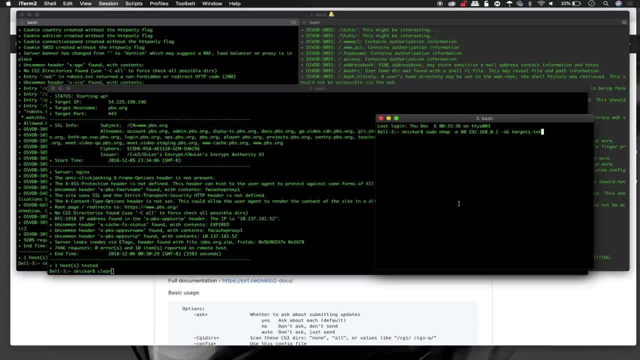 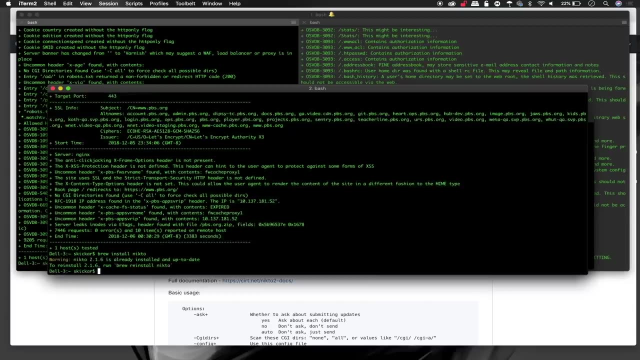 and if you're using Mac OS, you can actually just type: uh, what is it? Brew install. if you have homebrew, which you should get And that should go ahead and install it for you. So, as you can see, it's already installed and up to date. 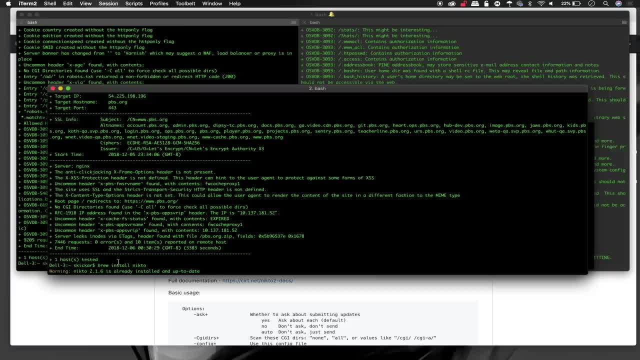 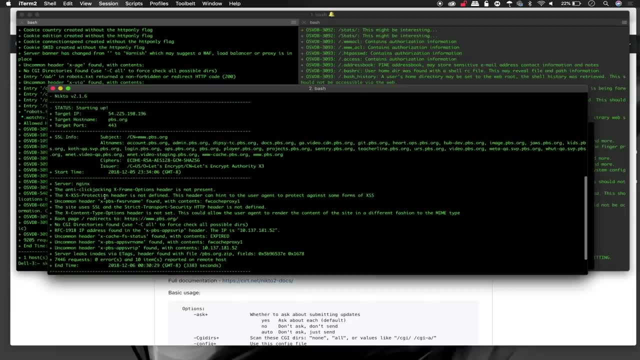 but there's a bunch of windows on my screen. All of these are results from Nikto scans and I want to go through them with you. so let's go through them one by one and see exactly what's going on. So, the first thing that's useful, which we'll start with: 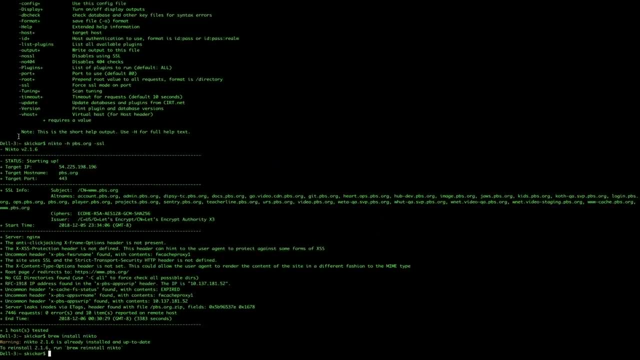 is the fact that Nikto is capable of doing a scan that can actually go after SSL and go after port 443.. So that means that, rather than being stuck to only the older websites, we can do vulnerability assessments on websites that are using SSL. 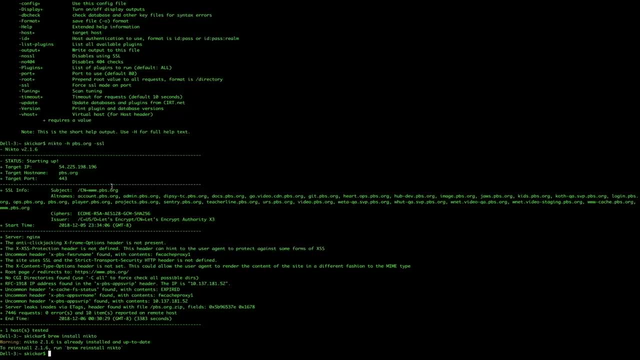 So that's great, and we can not limit ourselves to some of the more vulnerable ones. Here we can see some Cypher information from the SSL port of pbsorg. Now the command to go ahead and run this is nikto tack h for host. 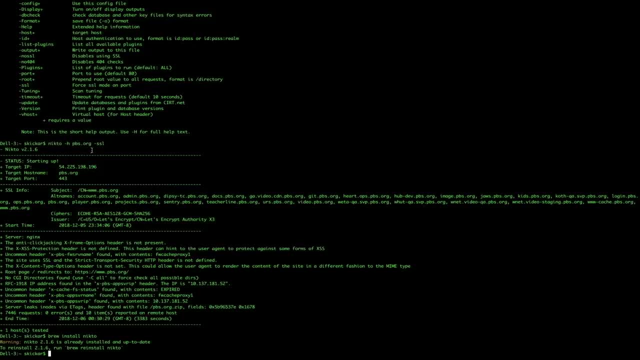 and then just pbsorg, And here we can specify tack ssl in order to speed up the scan and let Nikto know that this is a SSL encrypted target. So once it connects on port 443, we can get this useful information about the Cypher. 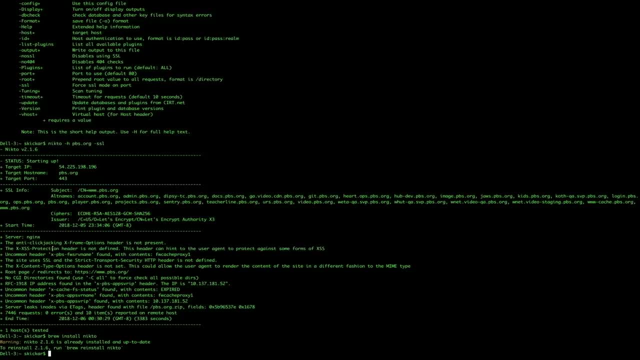 and a list of other useful details that Nikto has found as it scans the website and defines certain pieces of information. So here we didn't find anything too earth-shattering, but this is a useful start. but that assumes, of course, that we already know the target that we want to go after. 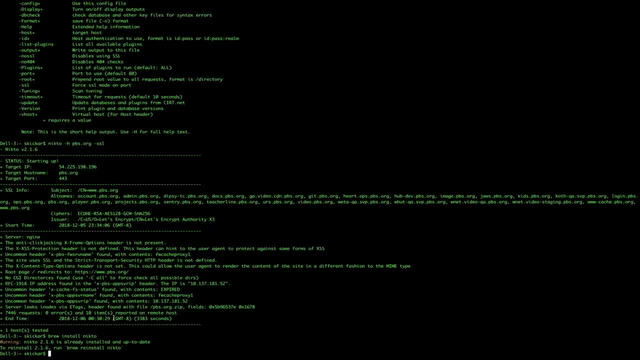 Let's go over another use case where we want to use Nikto on a local network to find embedded servers, like maybe a login page for router or something like that, and maybe discover vulnerabilities on our local network. Well, let me clear the screen. 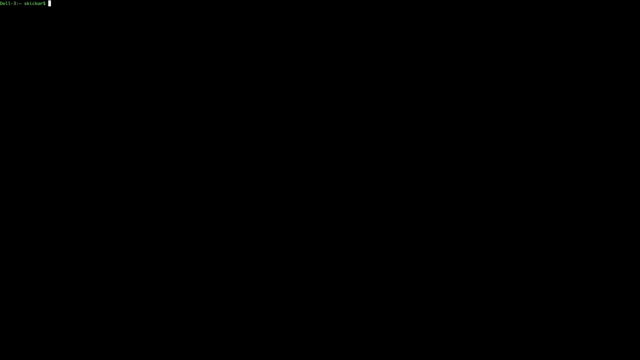 And the first thing we'll need to do is actually discover exactly what we have going on on our network and which devices will be vulnerable to maybe something we have on the web application side of things, meaning a port 80, a port 443,. 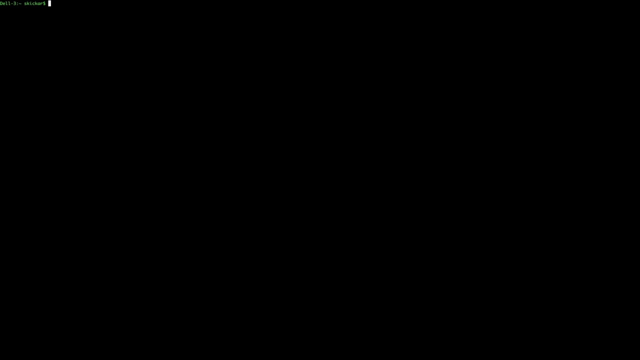 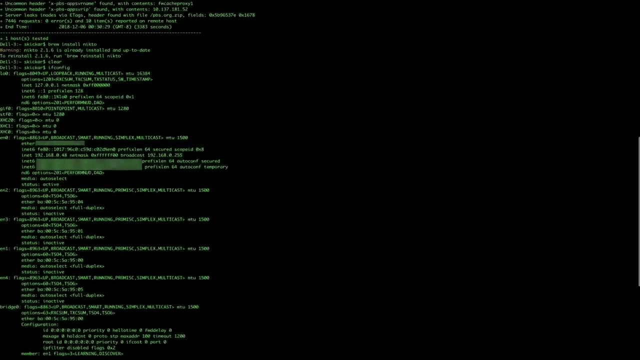 or something else we might expect a web server to be running on. So to start, let's get our IP address, We can type ifconfig And then, once we have our IP address here, on our iNet interface here we can run ipcalc. 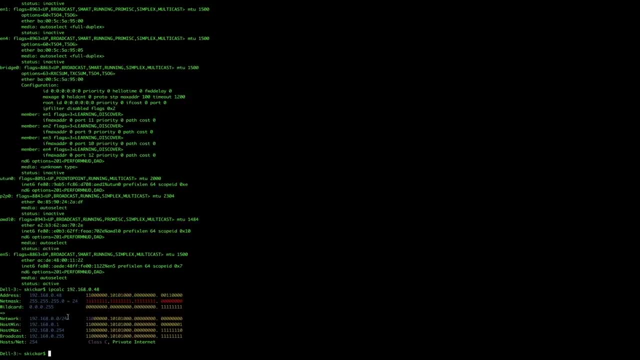 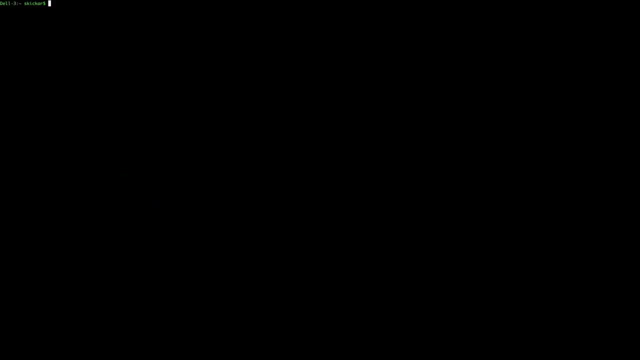 to get our network range if you're a beginner and you don't want to actually do it yourself. And boom, we have the network range. So we can now run nmap. but let's make this a little bit easier for ourselves. So if we're going to run nmap, we can do nmap tackp for port 80,. 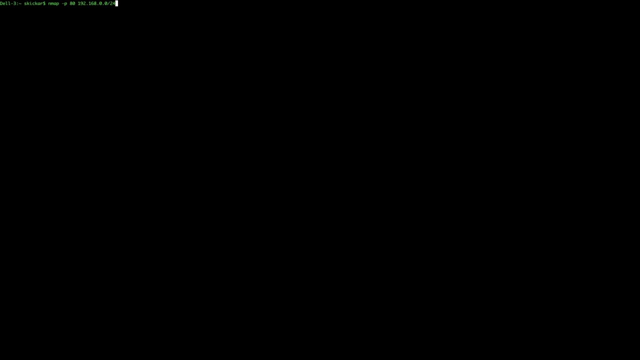 and then we can specify our host range as we normally would. But we want to make this easier to work with, to just extract kind of the hosts that are up, aka the ones that are responding and saying that they have port 80 open. 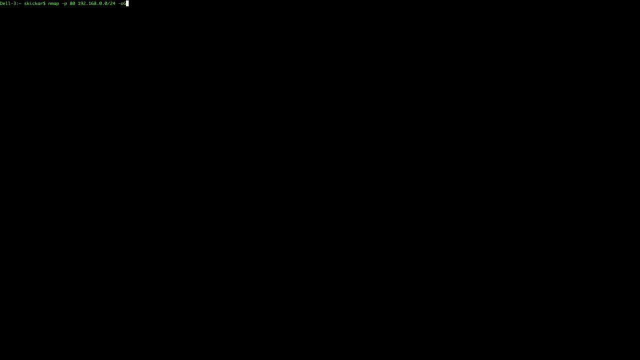 So we're going to use the lowercase o, uppercase g, grippable output and then make a file called, let's say, nullbytetxt. So this will go ahead and run our scan and save it to a file. but we can use a nice little trick here to make it easier for us to go ahead. 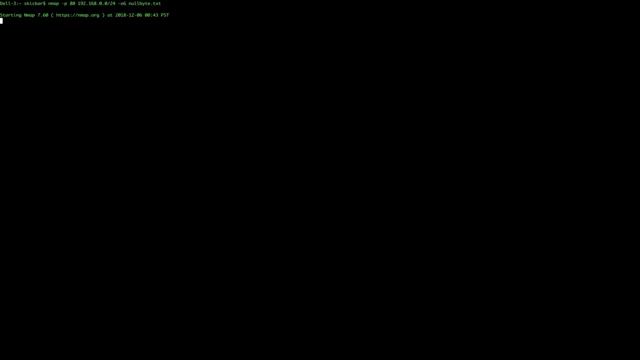 and locate anything on the network. So we're going to go ahead and do this by IP address and just pass that to Nikto so it will automatically attack it. Now, that's a lot of information and this is fine, but we can see that there are a couple of these hosts. 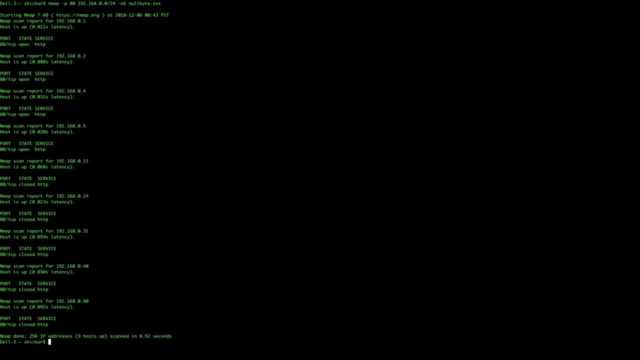 that are reporting themselves as up. What can we possibly do to make this maybe a little bit more convenient for Nikto to go through? Well, it turns out there's a command we can use that is really helpful, and I want to show you guys what it is so we can use it. 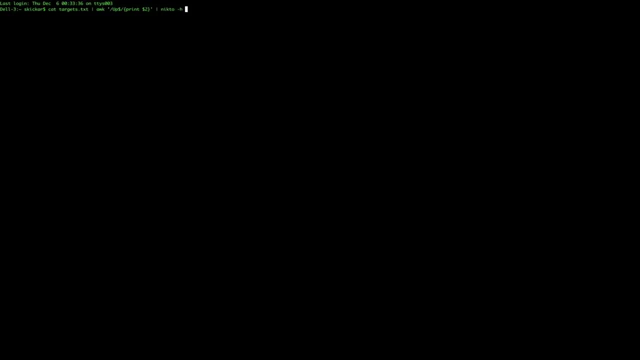 So here we can see a command that's pretty useful, and what we're actually going to do is take our nullbytetxt and replace it with, for the example, targettxt, And what we're going to do is basically say cat, nullbytetxt. 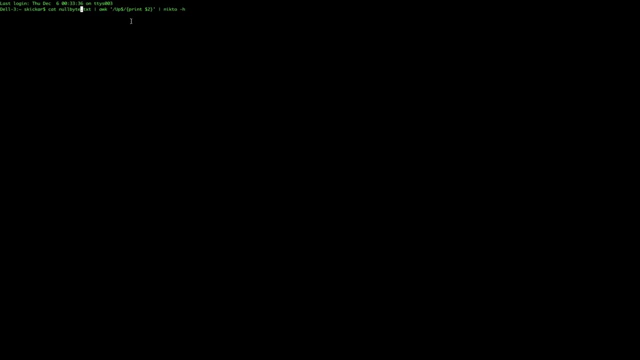 so read out the contents of nullbytetxt that we just saved, which is all that nmap scan saved in a special format. and then we're going to use this Linux tool, awk, to search for a pattern of basically up saying that a host is up. 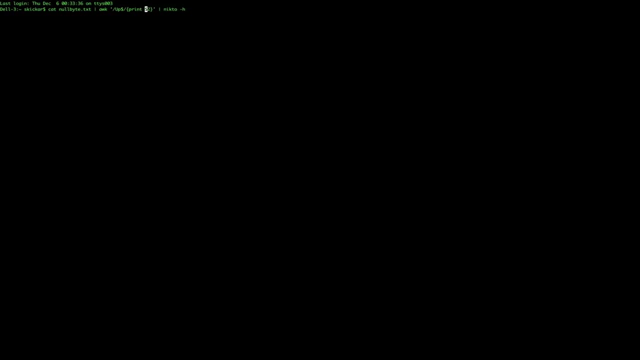 and then print out the second word in that line. So this is going to be just the IP address, and that'll be nice because in the end that'll allow us to create a file which we can type cat, called targetiptxt. 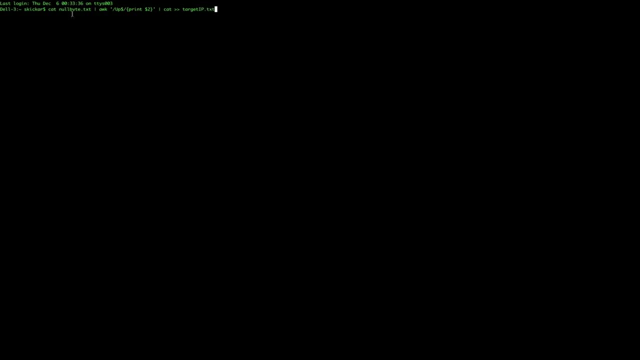 So again, what we're doing is we're reading out all this contents of the nmap scan we just did, We're using awk to search for this pattern and then print the second word in that line and then we're taking just those IP addresses. 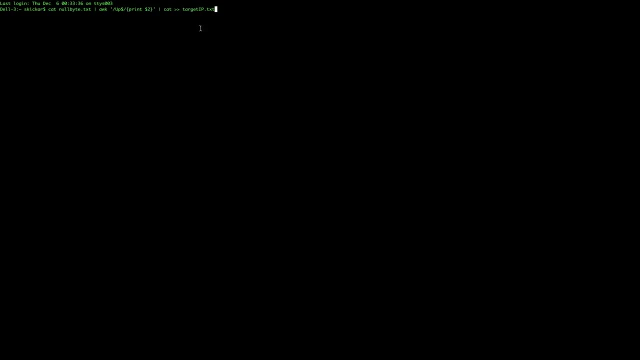 and putting them into a file called targetiptxt. So when we run this, we can now cat targetiptxt and boom, We have a list of all the IP addresses that say they have a port 80 running. So this is perfect for Nikto. 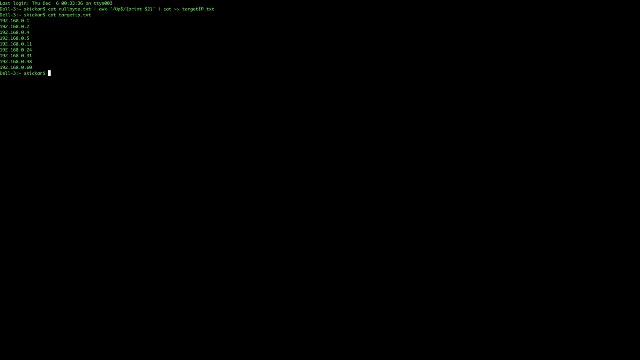 because it's capable of easily interpreting files like this. So now we can simply run Nikto and then targetiptxt, And now Nikto will run against all of the various targets that we've specified in this file, which is a pretty fast and easy way of going after. 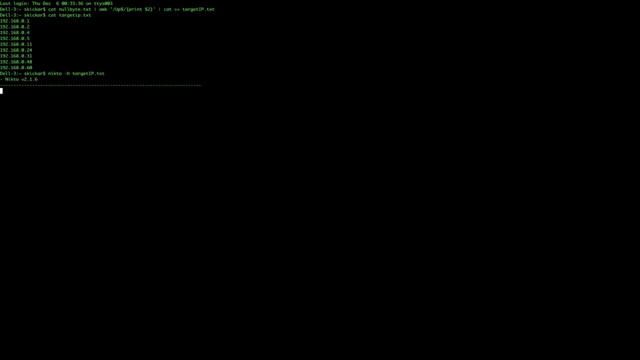 pretty much everything that has a port 80. open on a local network. Now you should take note that Nikto does take quite some time to scan on occasion, depending on your connection speed and how fast the target is responding. While this scan runs, I'm going to go ahead. 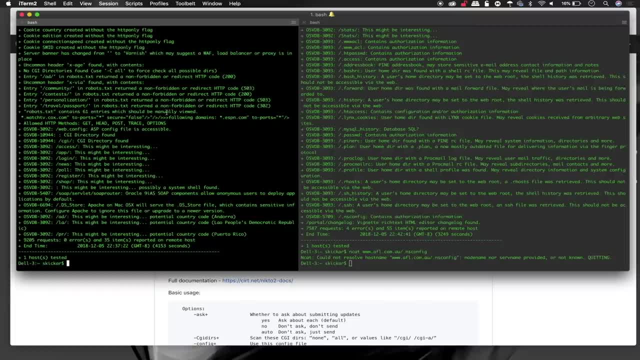 and show you some of the other scans I've already recorded so you can see what some of the results look like when you go after the two other types of targets. Now we've shown what it looks like to go after an IP address and also what it looks like to go after a SSL target. 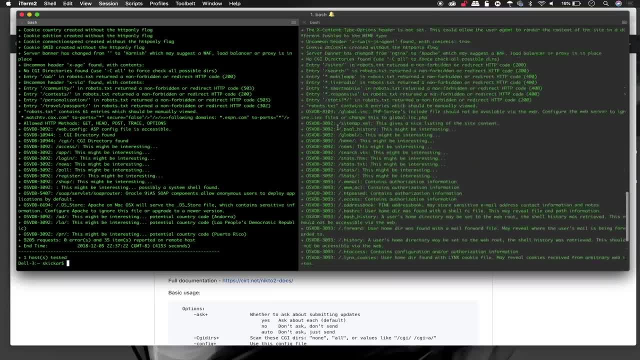 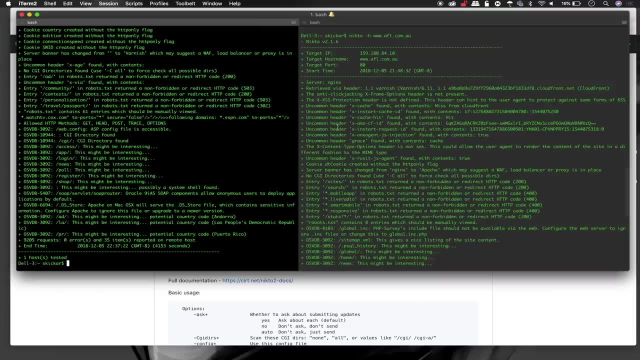 So if you're going after a simple website that just uses port 80 and doesn't have HTTPS enabled, then you can get a lot of really useful information. So let's take a look at one of these outputs here Now. I followed a link to a website. 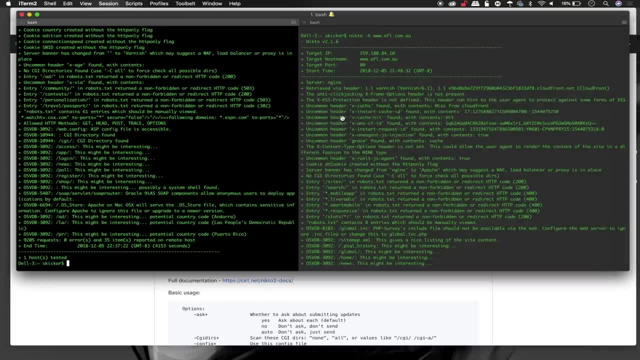 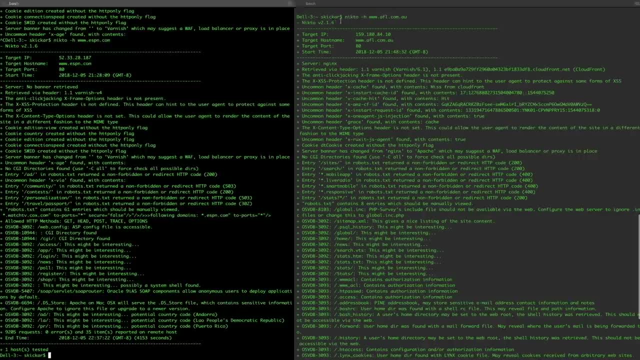 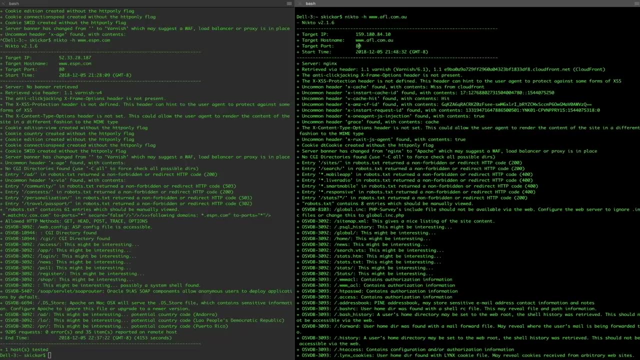 that was just about all the different major websites still using HTTP and not HTTPS, And one of the biggest in Australia anyway is the Australian Football League. So that seemed like a good website to test out, So I just typed: Nikto tack H. 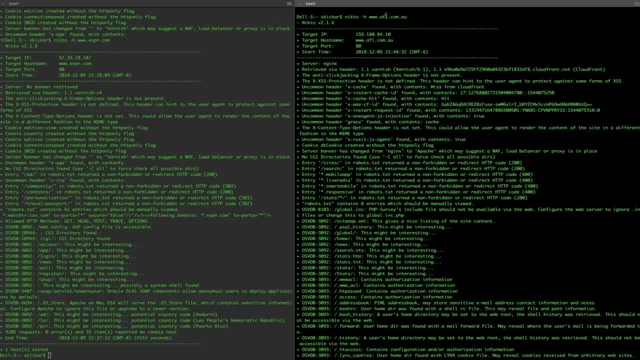 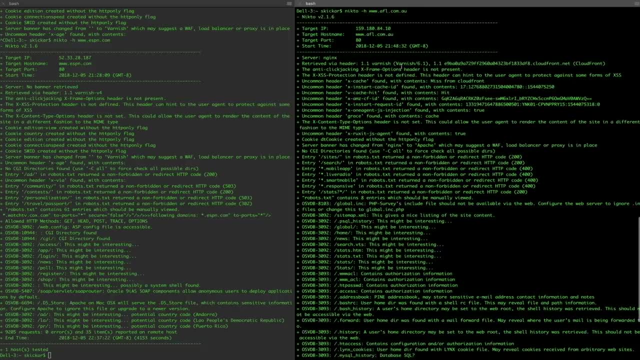 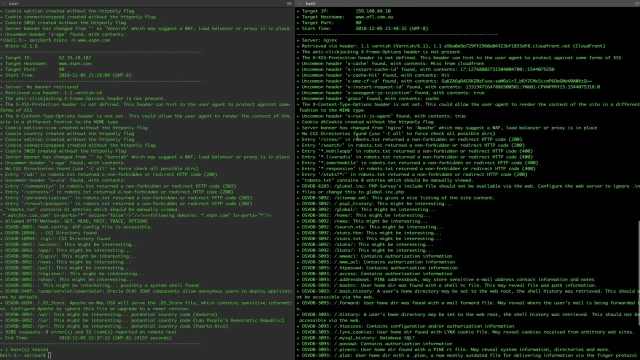 and then wwwaflcomau and we get an IP address and Nikto just goes to work. So immediately we can see we have a Varnish server that we're working with and then some other information about headers which could give us some information. 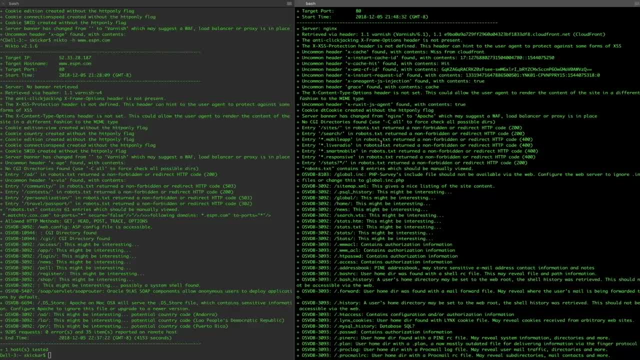 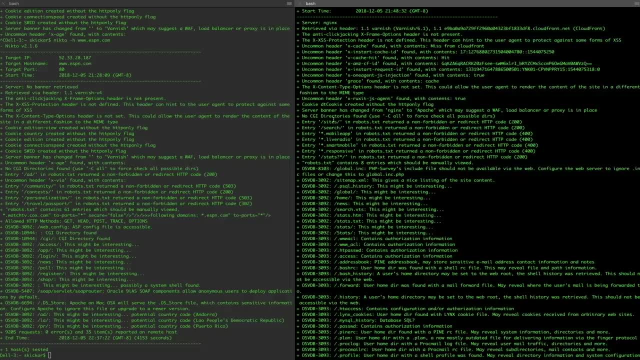 about the way that the website's configured, But really the more juicy stuff is finding directories which allow you to start even pulling down the configuration files, which might contain credentials or other things that have been misconfigured and unintentionally left able to be accessed. 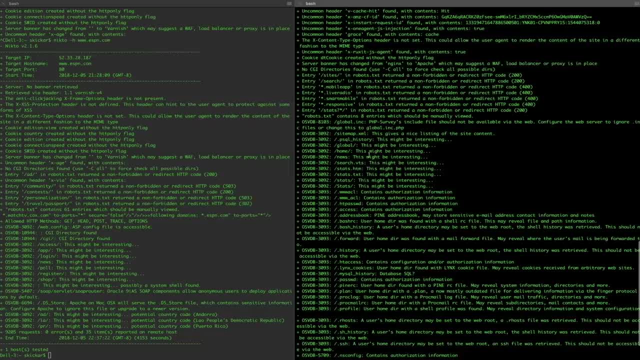 So here we can see, there's a number of observations that seem to imply that going to these different subdomains or folders may be interesting, And as we explore them, I was able to see that a couple of these actually do allow you to download configuration files. 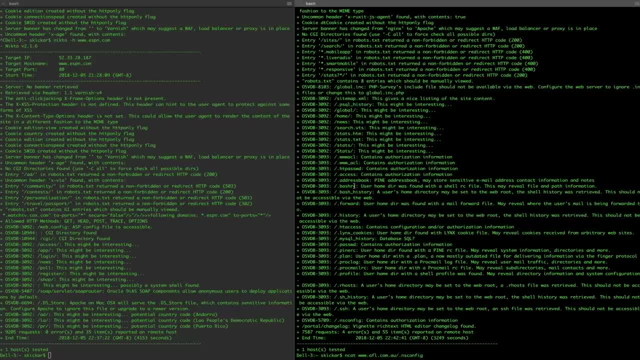 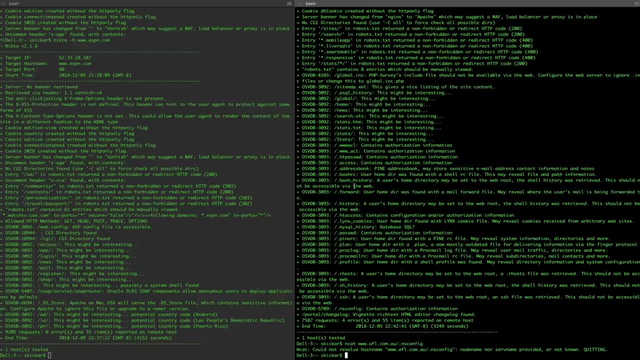 for the website, which probably almost definitely should not be public Now. we didn't find any critical votes or vulnerabilities, but I'll show you what we would do if we had, because this is really the step where Nikto would go from simple and rather active scanning. 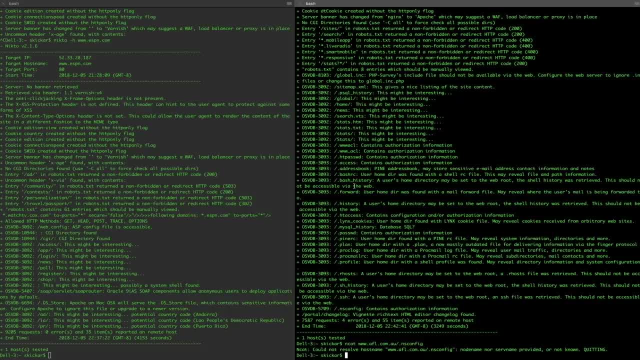 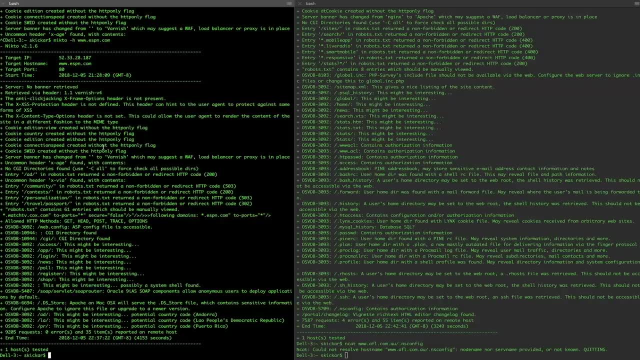 into actual expectation, or at least the planning of something a little bit more direct. Now we can see in the United States version of ESPNcom we actually don't find a lot more than we found on the Australian version, but it doesn't mean that we can't show you what we would do. 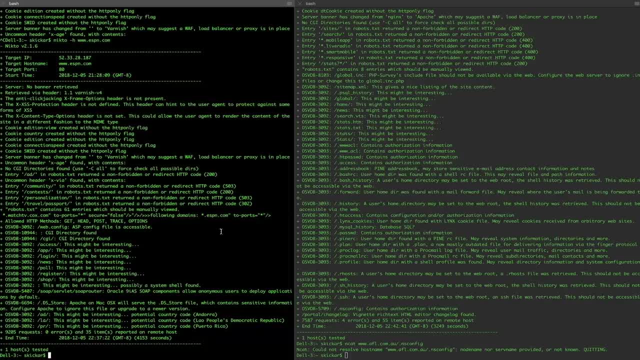 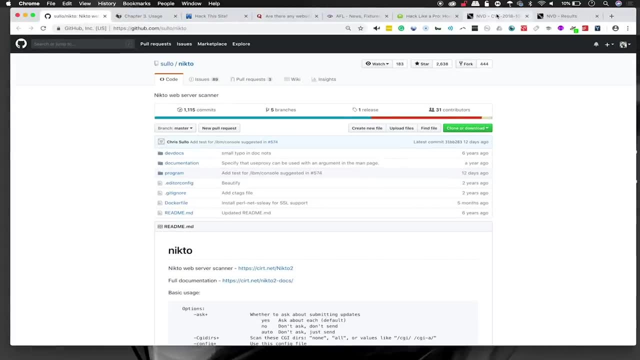 had. we found a critical vulnerability on a website, So in order to actually use this, we would need to pair it with an exploit, And when we go back to a website like the National Vulnerability Database, we can plug in anything that Nikto gives us. 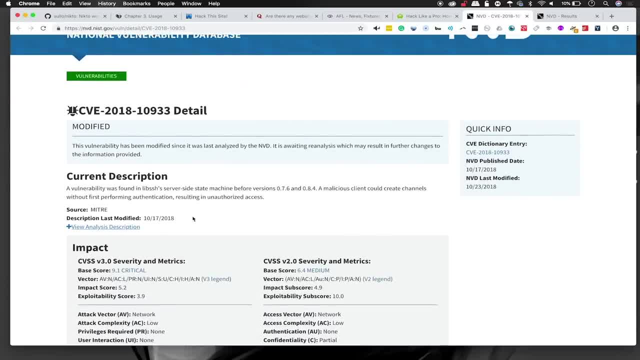 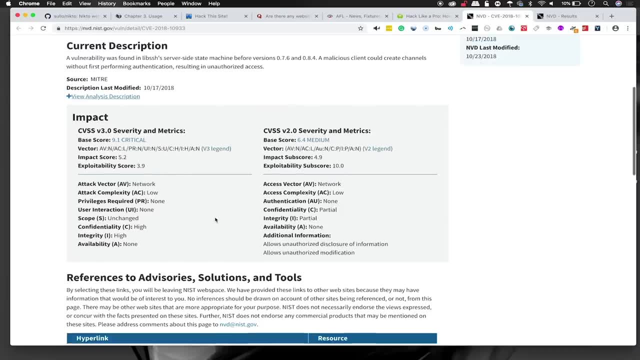 and come up with a CSV detail file which shows us more information about the vulnerability. Here we can see that this vulnerability is rated as critical. It has a medium base score. We can see that the attack vector is over network low complexity. 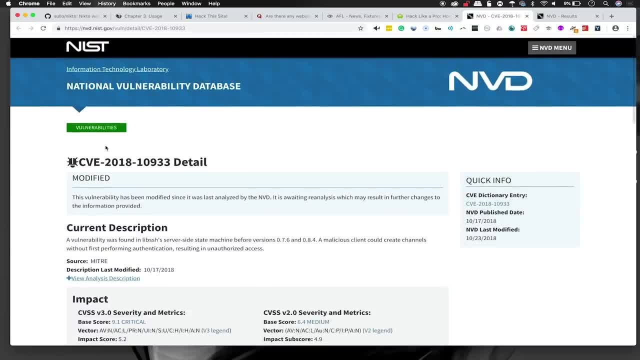 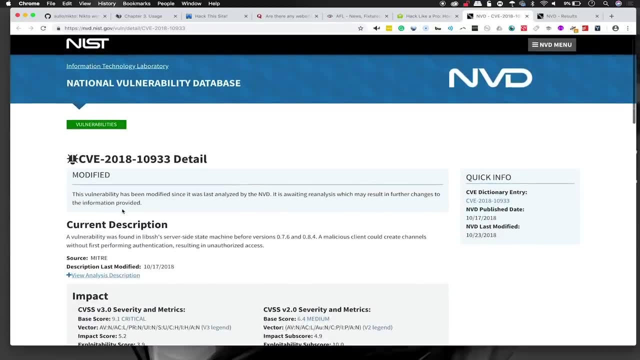 pretty much anyone can do it, So of course, this is a previous one. we reported on the leave SSH vulnerability, but a CSV file will look pretty much the same for any CSV that you find, which is a critical vulnerability on a network that Nikto recognizes and reports back to you. 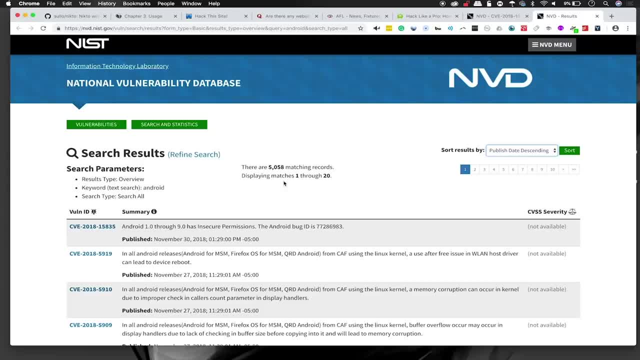 So the last step of this is pairing one of these results, which you can access through just a simple search on the National Vulnerability Database website, with an actual exploit that someone has weaponized. Now, if you're lucky, there can already be a module for this in Metasploit. 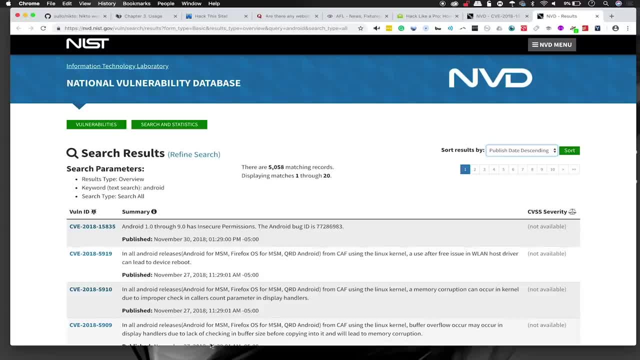 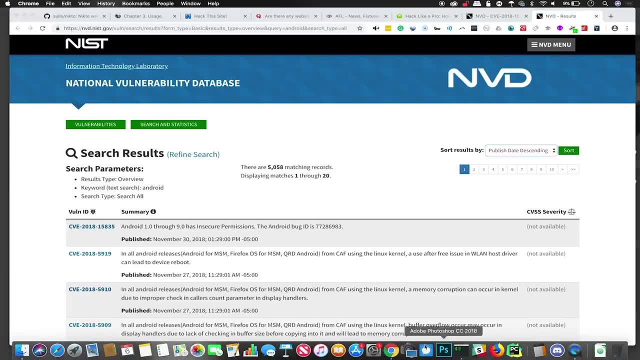 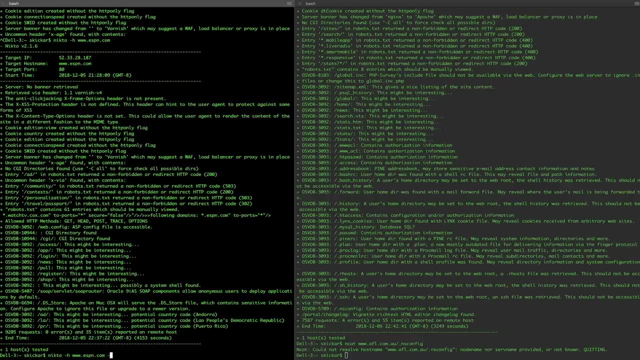 And you can even export things to Metasploit from Nikto or at least put it in the right format so you can just open it up in Metasploit by just typing when you're doing a Nikto, scan Nikto, and then adding the additional flag. 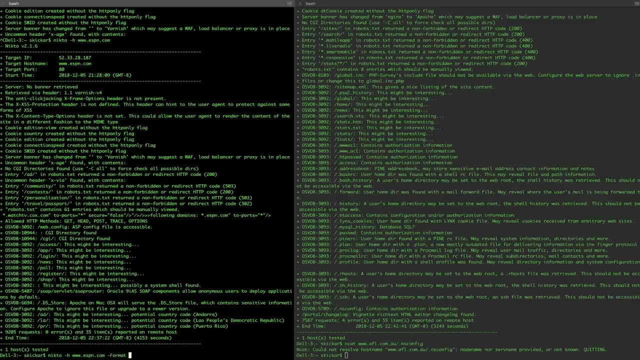 format, and then msf plus. Now again, the reason this is useful is because, by appending this to the end of our Nikto command, we're able to save this in a format that will quickly pair it with, potentially, a weaponized exploit. 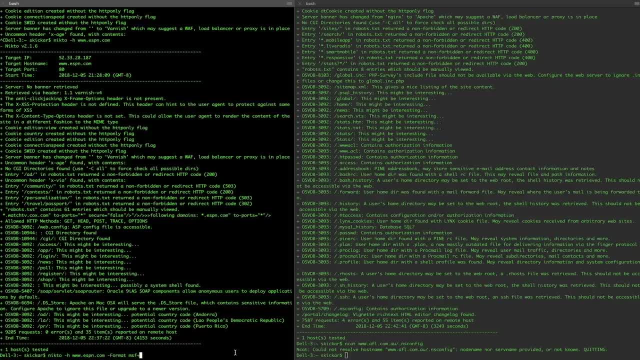 kind of closing the loop and going all the way from detecting the target surface area, finding a vulnerability and then pairing it with a weaponized exploit, so we don't have to do all the work Now, before you start running Nikto on every website you can think of. 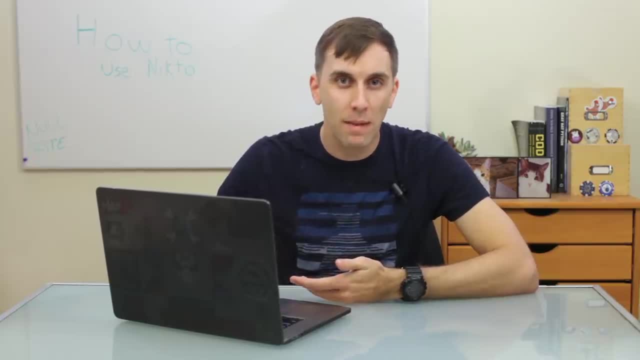 it's important to understand that this is quite different from something like an Nmap scan. While a basic reconnaissance scan is usually perfectly fine to do, if somewhat noisy, a Nikto scan can go a lot further and exhibit some behaviors that could be flagged.